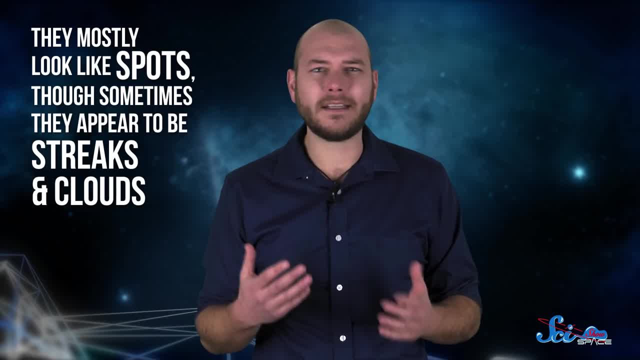 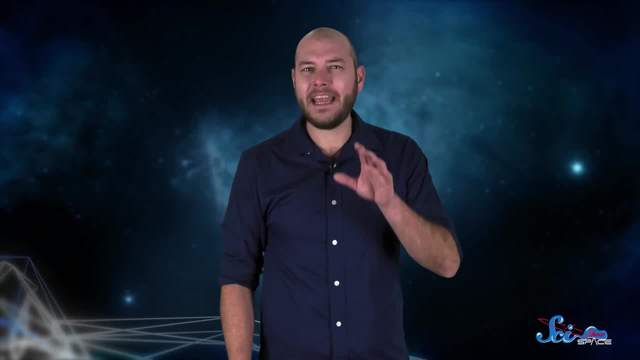 The Apollo astronauts who first described them said they mostly look like spots, though sometimes they appear to be streaks or clouds. They were bright enough that they even kept some astronauts awake at night. By taking a close look at the Apollo astronauts' helmets, 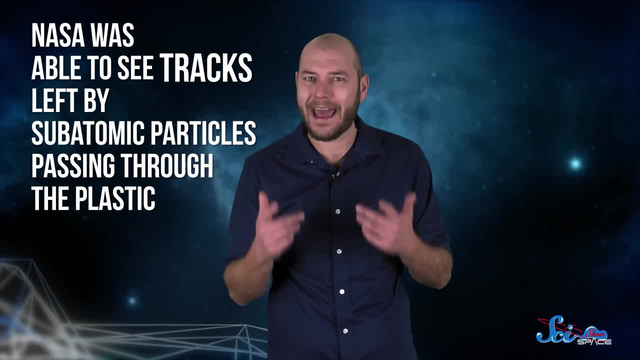 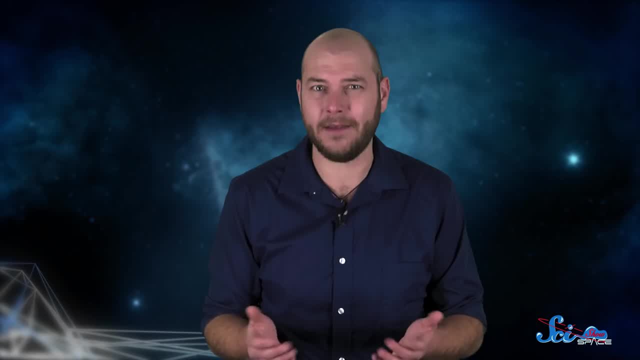 NASA was able to see tracks left by subatomic particles passing through the plastic, And in the 1970s some ground-based scientists conducted some maybe-not-so-super-safe experiments. They had people look at a neutron beam in dark rooms which caused similar flashes to appear in their vision. 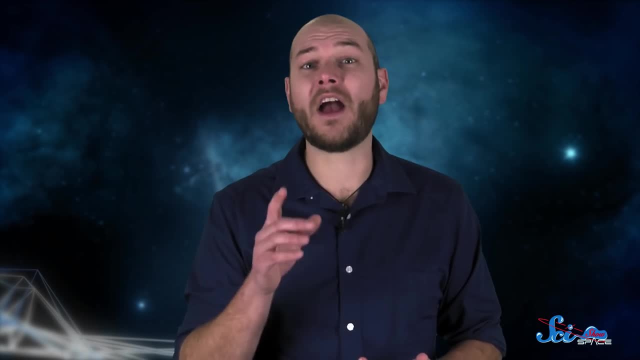 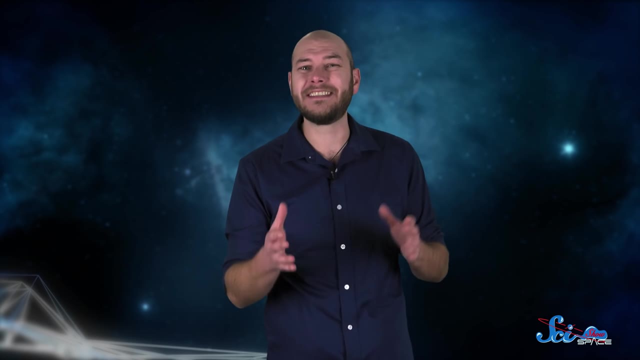 Some more modern astronauts are outfitted with special helmets with cosmic ray detectors. The astronauts keep track of when they see a flash to collect data on what types and energy levels of particles seem most likely to cause them and how often they appear in different employee spaces. 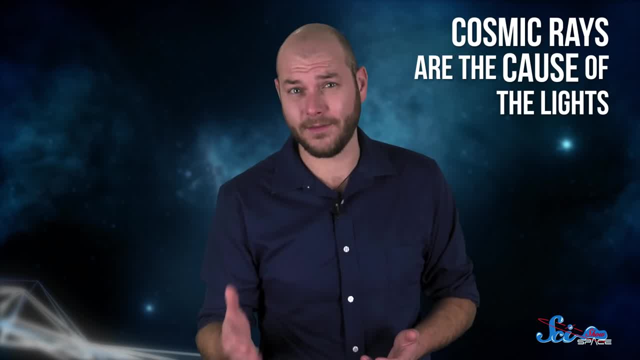 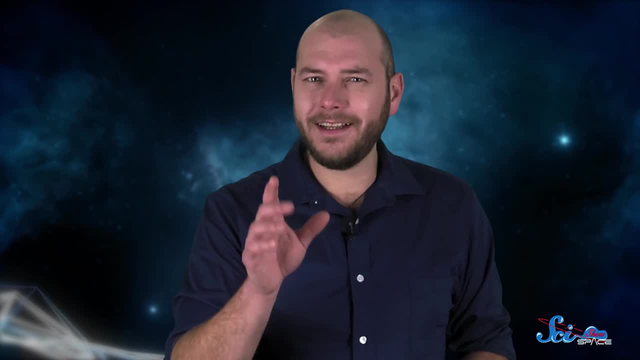 different parts of space. So we're pretty sure that cosmic rays are the cause of the lights, and researchers hope to use these data to come up with better ways to protect astronauts from cosmic radiation. But there's still a big mystery. We don't really know what's happening inside astronauts' eyeballs when these flashes. 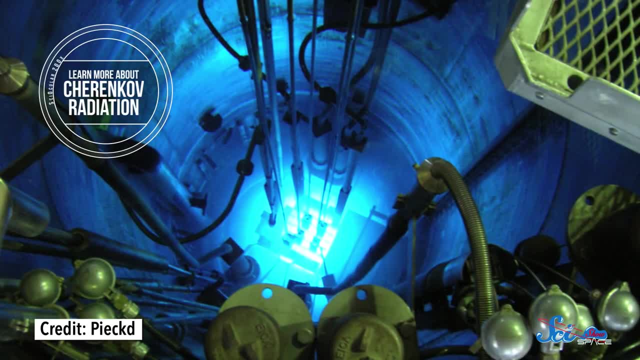 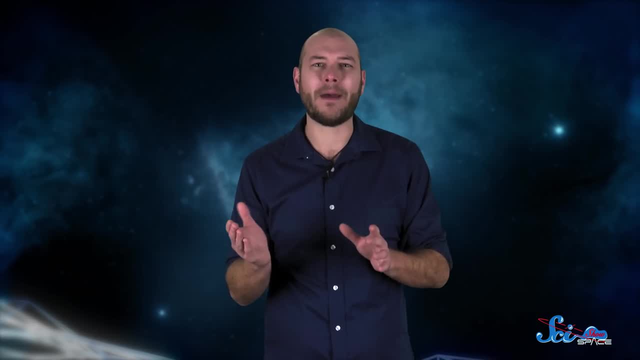 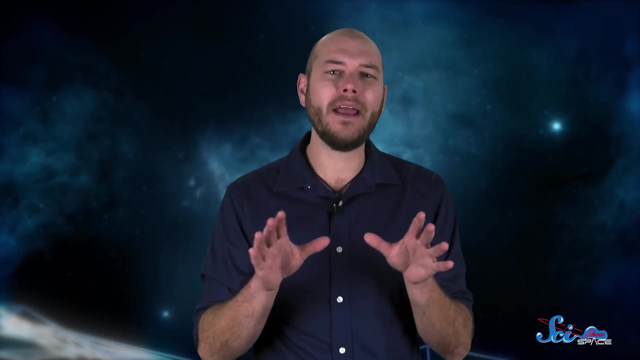 occur. One possible culprit is Terenkov radiation, which causes the blue glow you might have seen in photos of nuclear reactors. Terenkov radiation happens when really energetic particles pass through a liquid faster than light can travel through it. These particles can interact with some of the liquid molecules which respond by emitting. 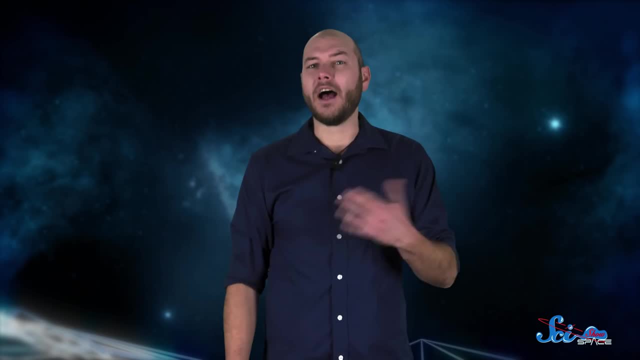 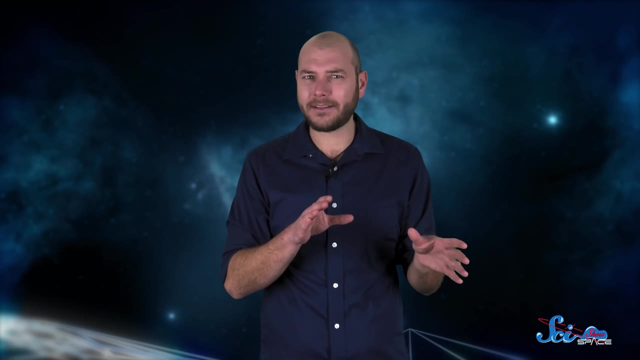 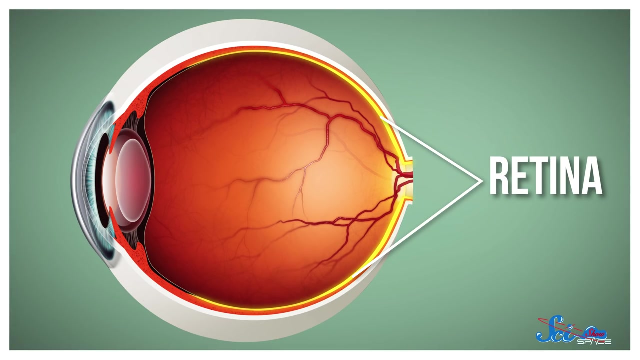 some photons of light, the glowing Terenkov radiation. Cosmic rays passing through eyeball fluid could be generating some Terenkov radiation, which astronauts see as spots and flashes. Another possibility is that radiation from cosmic rays could interact weirdly with the retina, the tissue at the back of your eye that normally detects visual light. 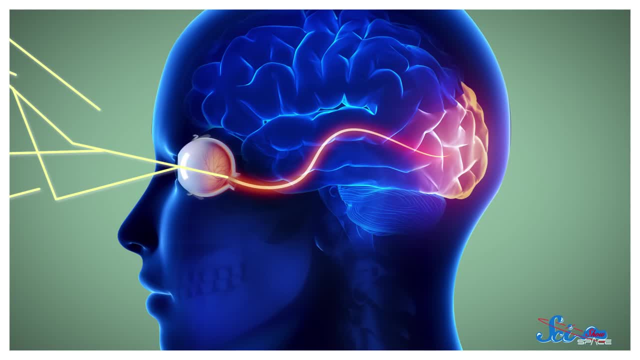 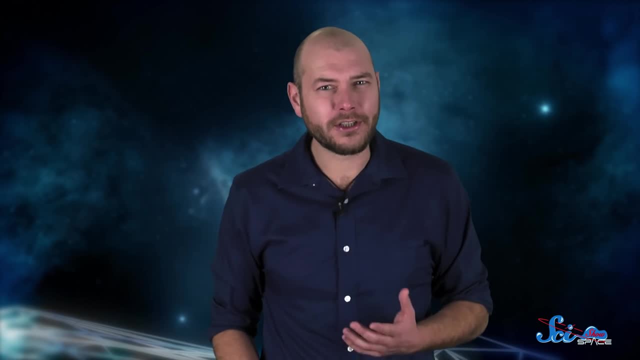 Or cosmic rays could bypass normal vision completely and pass right through the eyeball, directly stimulating the optic nerve or even the brain's visual cortex. Scientists still aren't totally sure what the right explanation is, since it's hard to do research on the eyeballs of busy astronauts in space. 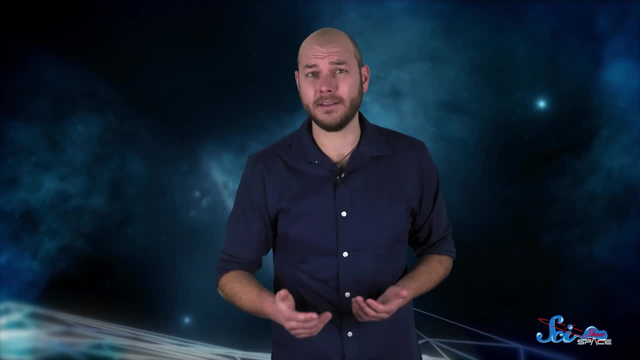 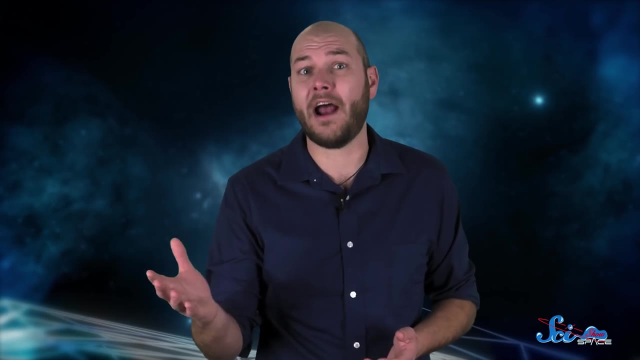 The flashes could even have multiple causes, which would explain why they don't all look the same. Cosmic ray visual phenomena are ultimately a pretty minor issue compared to being smashed by meteors or fried by solar flares, but they are a possible indication of damage to the.